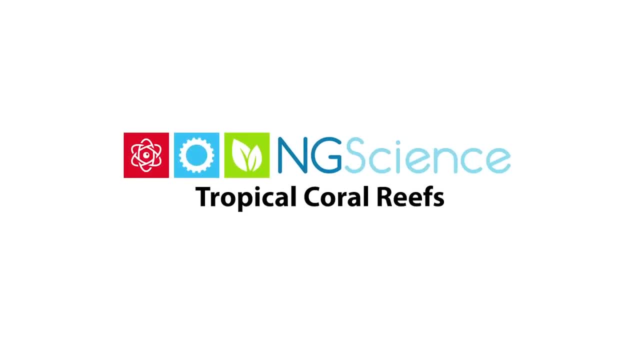 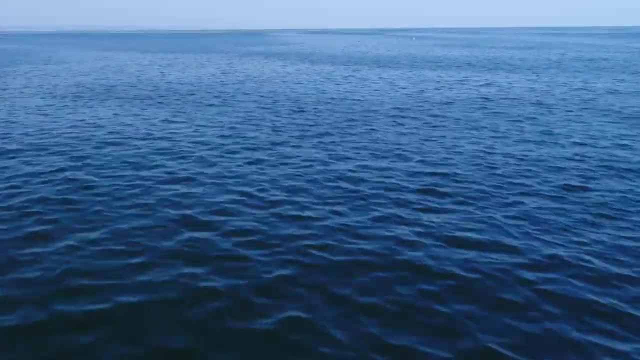 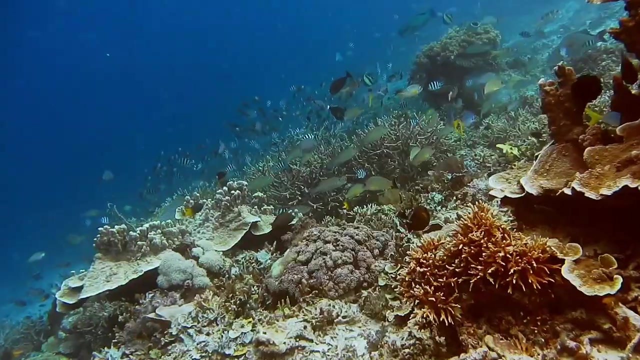 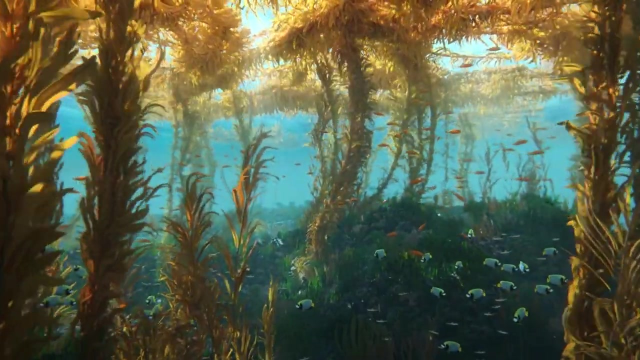 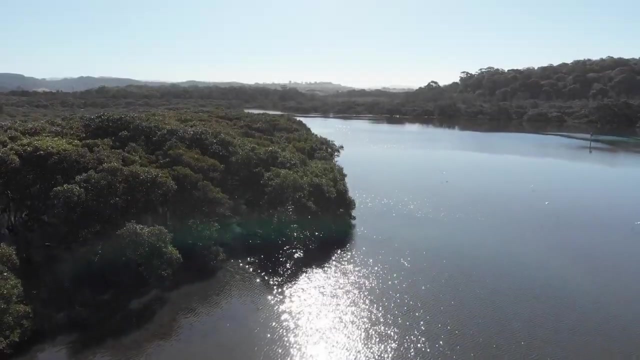 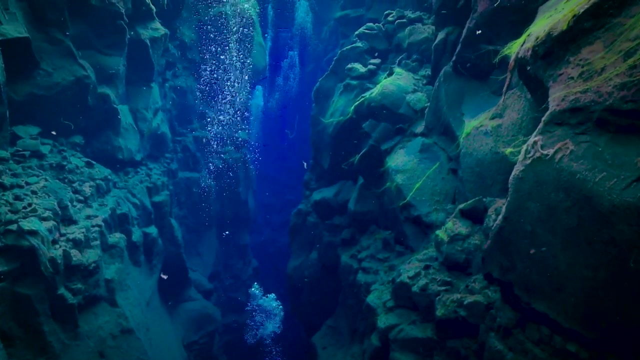 The ocean is a large body of salt water that covers more than 70% of the Earth's surface and gives the Earth its deep blue colour. Within the ocean are a range of different ecosystems: There are temperate kelp forests, mangrove forests, estuaries, open ocean and deep-sea ecosystems. 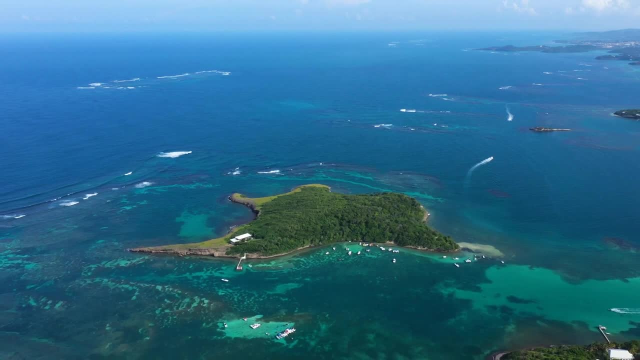 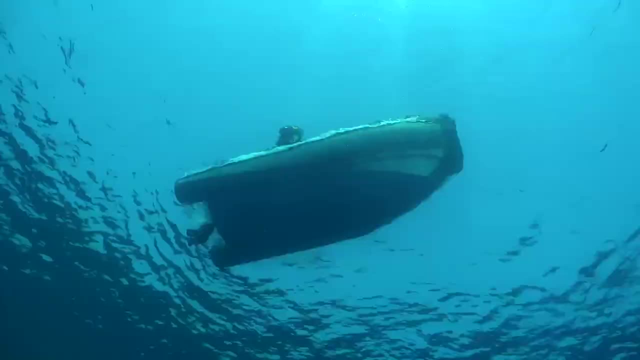 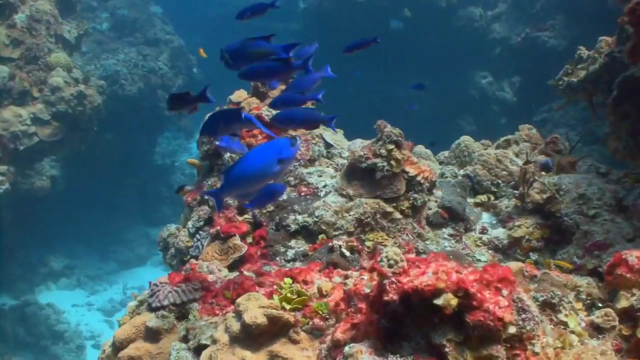 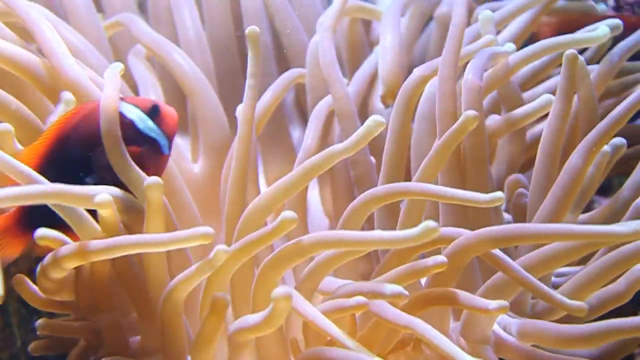 Today I am going to show you the most ecologically diverse ocean ecosystem of all – tropical coral reefs. Ready, Let's go. Tropical coral reefs are composed of colonies of marine invertebrates. Some corals, like anemones and sea fans, are soft corals. They have soft, flexible. 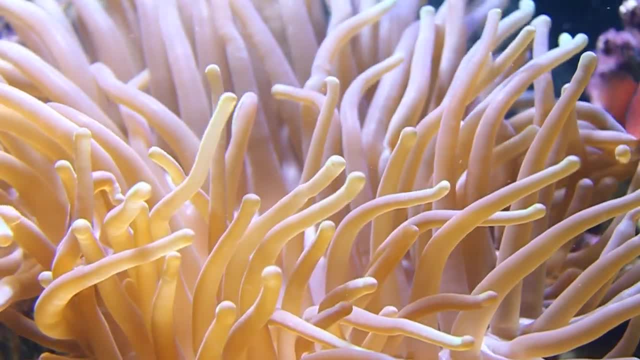 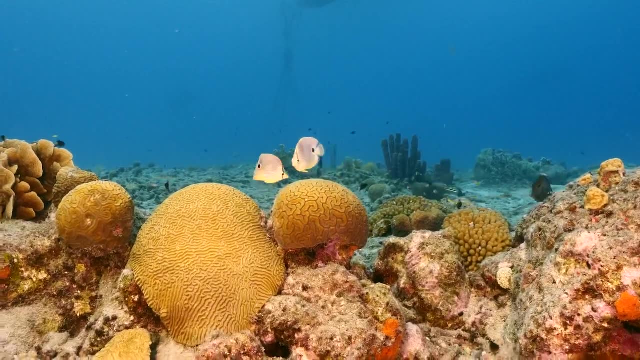 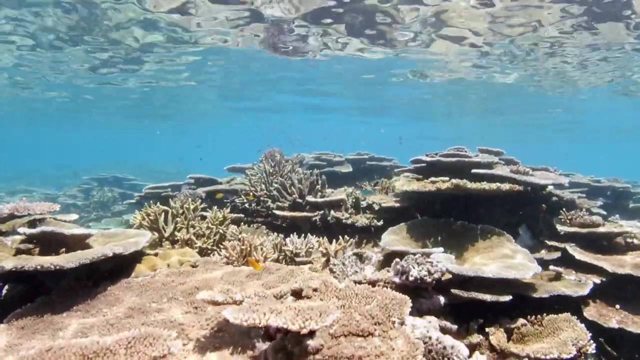 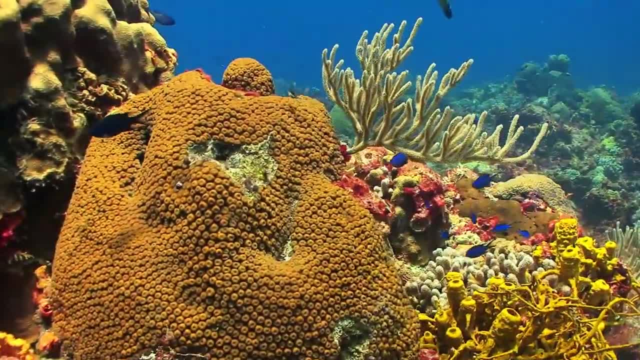 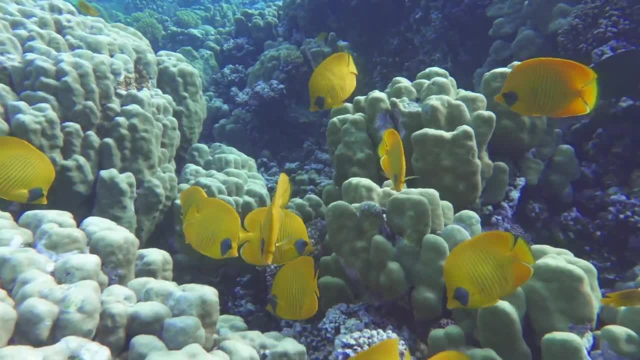 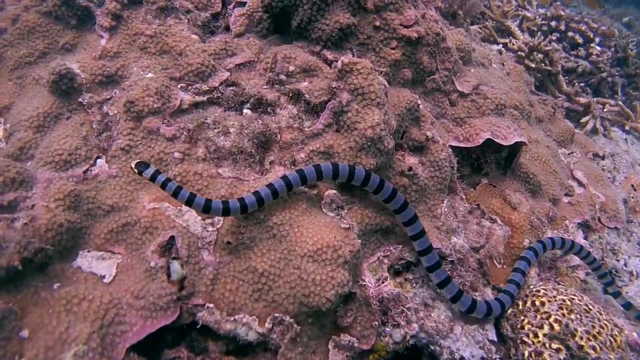 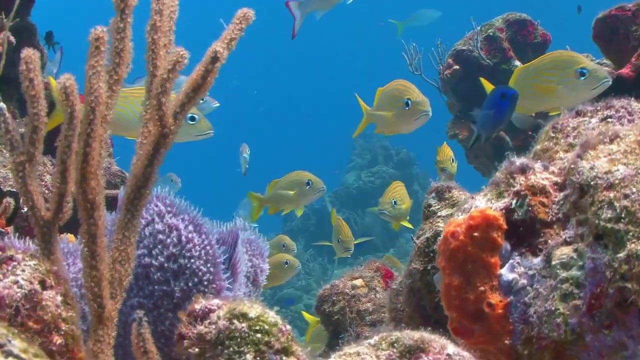 and grow Over hundreds of years. this process builds a coral reef. Coral reefs are underwater ecosystems that provide many habitats for a huge diversity marine animals to seek shelter, find food and reproduce. They account for less than 0.1% of the world's ocean area, yet are home to more than 25%. 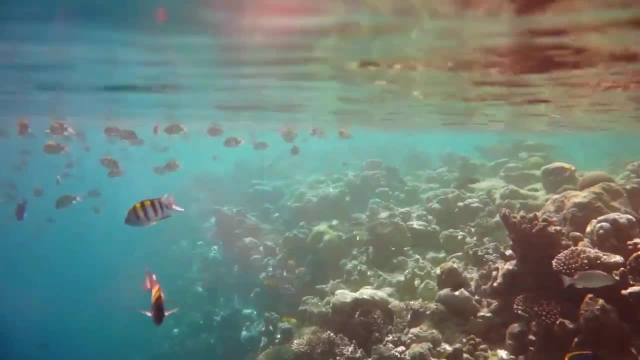 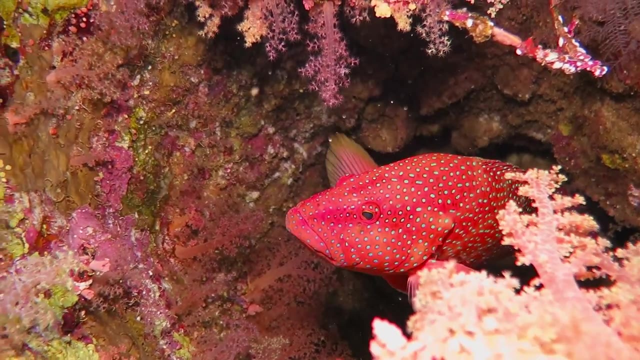 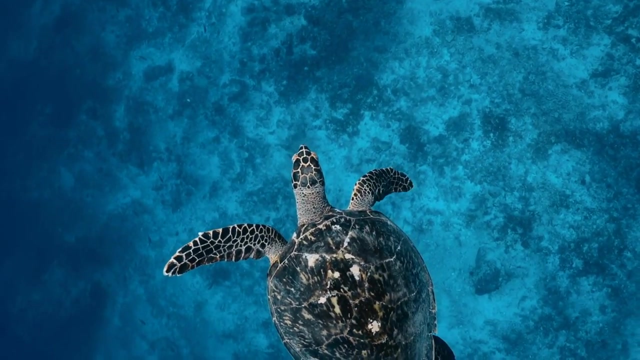 of all marine organisms. There is a great variety of fish, from tiny anemone fish and seahorses to fish giants like gropers, reef sharks and rays. Marine reptiles like sea turtles and sea snakes also cruise coral reefs in search of food.